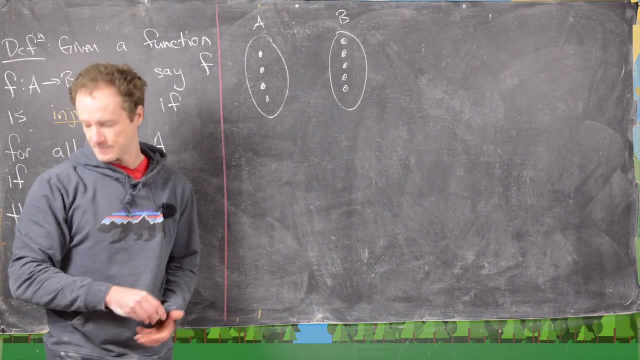 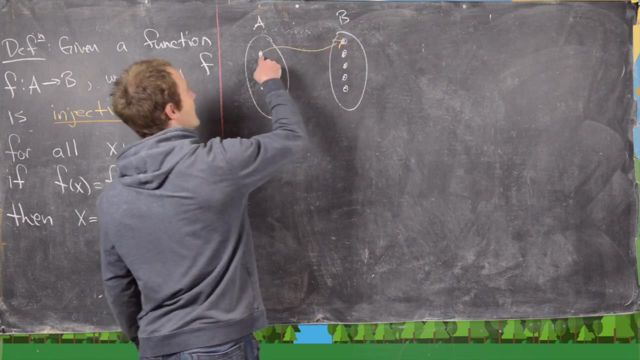 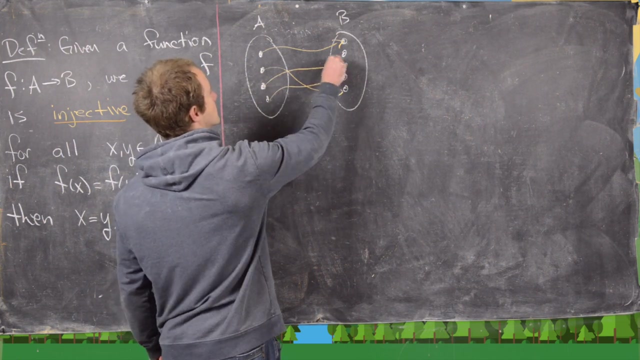 here that represent elements in b, and then we can draw our function as arrows from the dots in a to the dots in b, So if every element of a goes to a new element of b, so like this, this would be f of x. 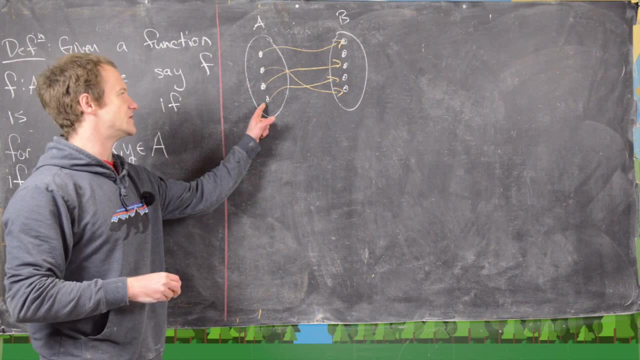 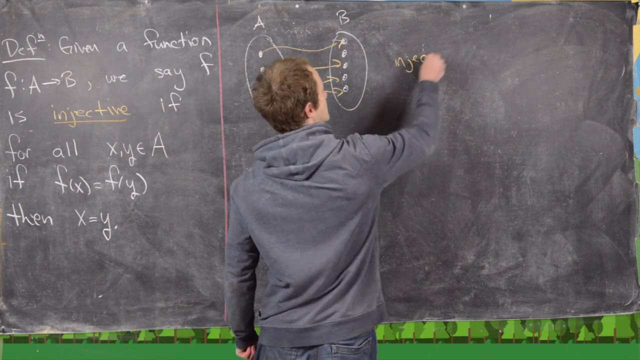 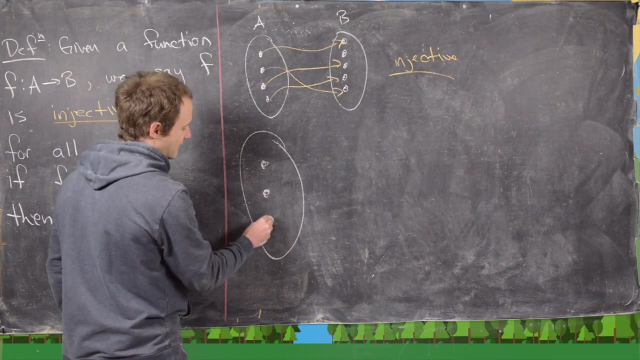 This would be f of x, an injective function. So notice, every element in the domain goes to a different element in the co-domain. So that makes this injective Good. But now suppose otherwise, that we have this function a? sorry, we have this set over. 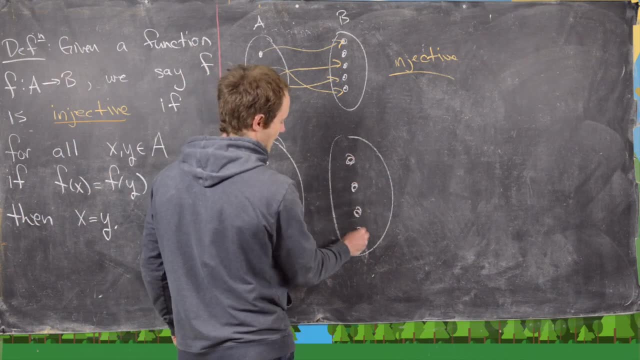 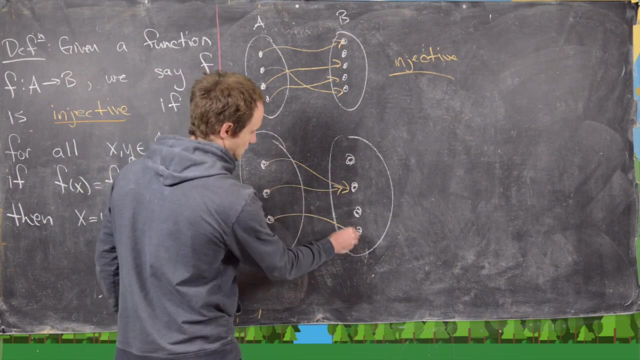 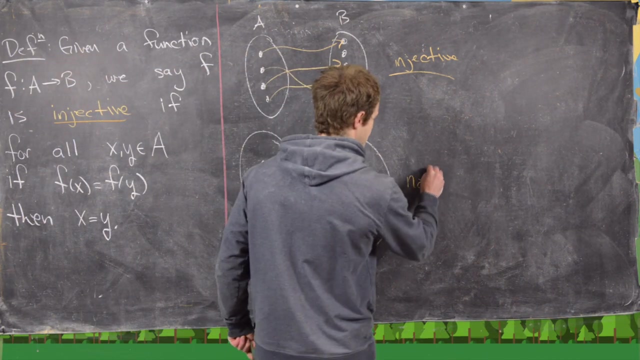 here a, which has these three dots, and this set over here b, which has four dots, and then maybe our function goes as follows: So these first two dots are mapped to the same element, so that makes this not injective Great. So now let's. 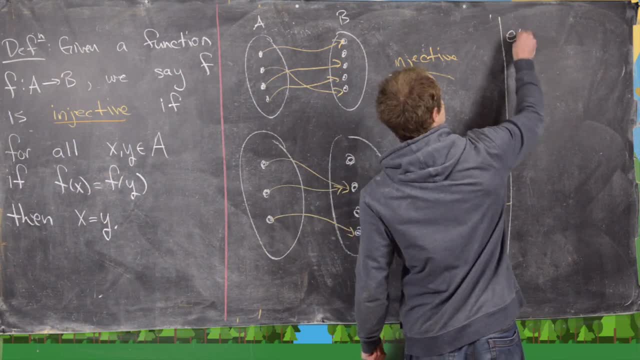 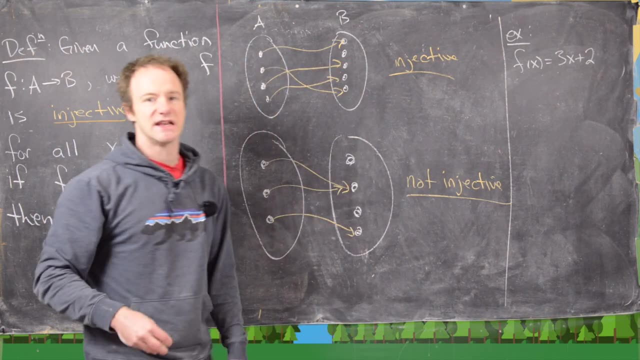 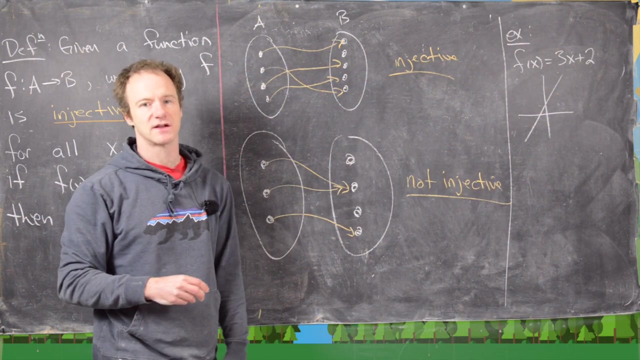 look at some examples that you will have seen, like in calculus class. So an example of an injective function would be like: f of x equals 3x plus 2.. So that's an injective function. notice that we could graph. it looks like that and that passes the horizontal line test and in fact, 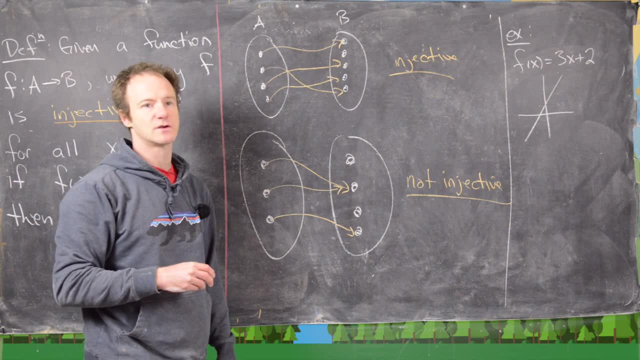 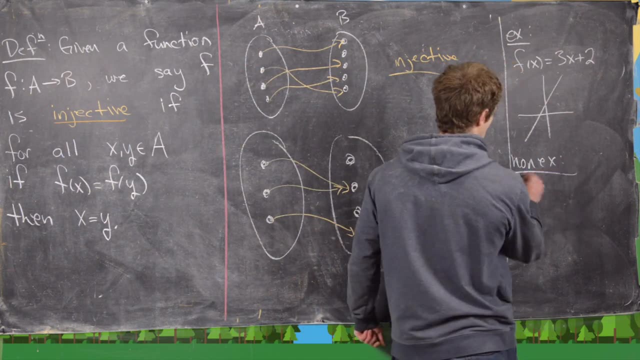 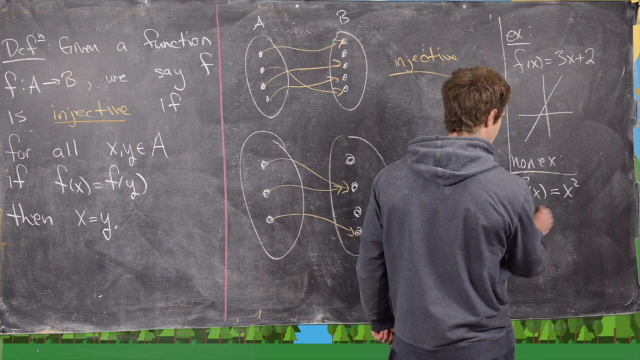 if you know the graph of a function, it's going to be inject over one to one if, and only if, it passes the horizontal line test. but maybe some non-examples would be like: f of x equals x squared, and that's kind of obvious because, notice, if we take f of negative one, we get one which is the. 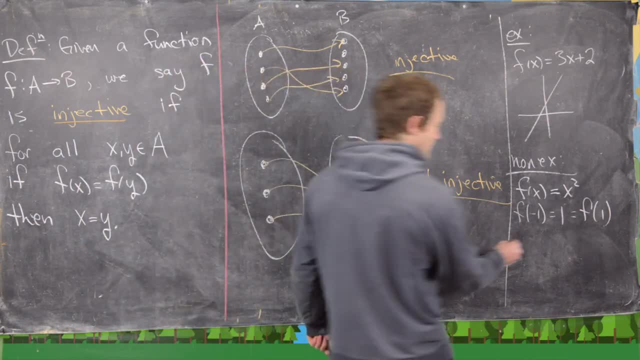 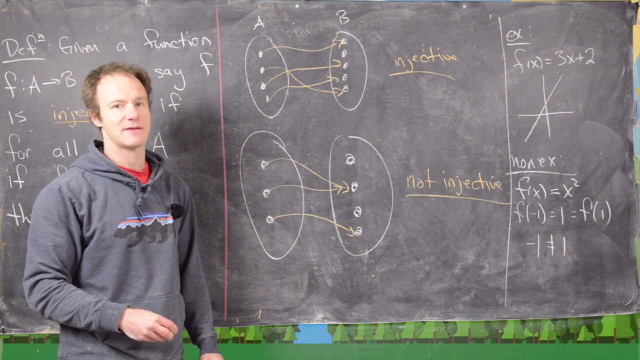 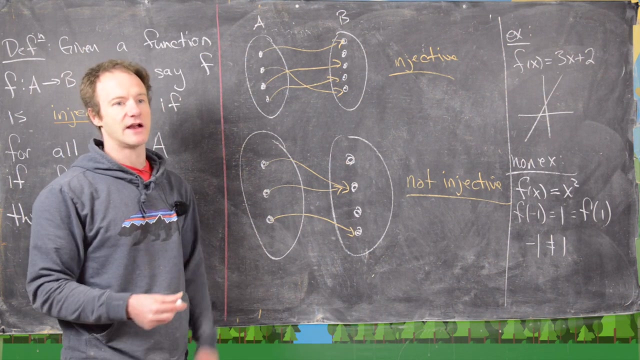 same thing as f of one, but negative one is not equal to one. in other words, we have two elements of the domain which are different, which are mapped to the same element of the range. okay, good, I'm gonna clean up the board and then we'll look at an outline for a proof approving something. 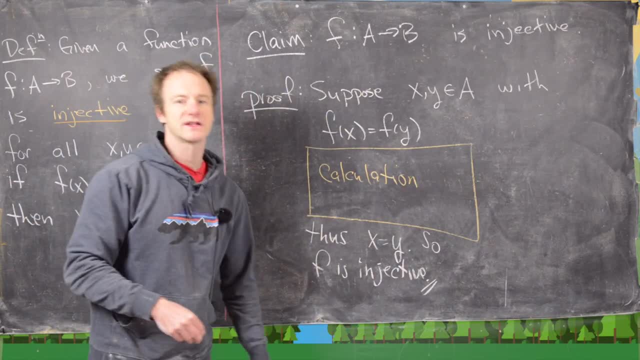 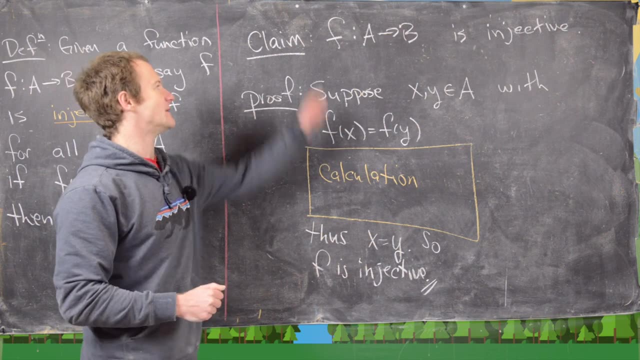 is an injective function. okay, before we look at some examples in detail, I want to look at the outline for showing that a function is injective. so let's say our claim is that this function, f from a to b, is injective. then the outline of, basically, 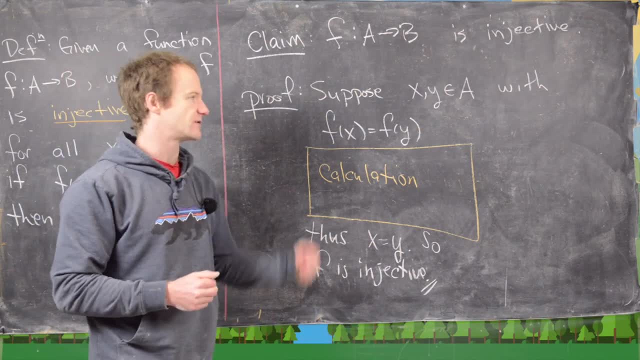 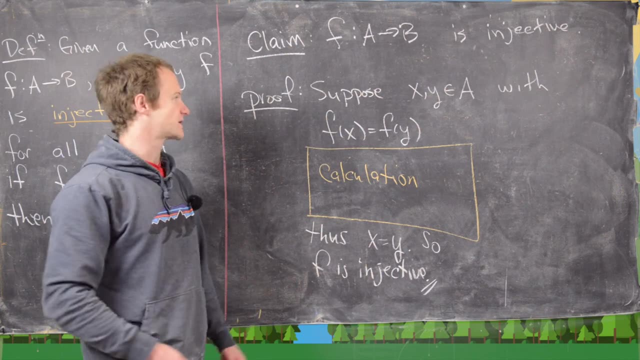 any proof that you would have to prove a function is injective looks like this. I mean, there will be some cases where it is easier to prove it another way, but this generally works. So you want to start off supposing that x and y are in. 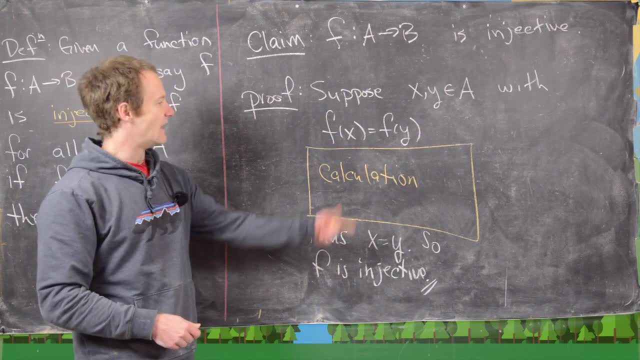 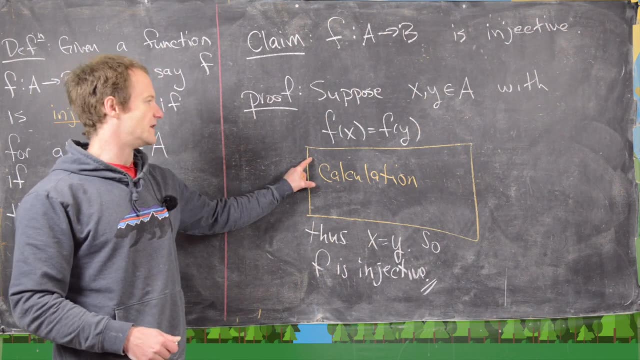 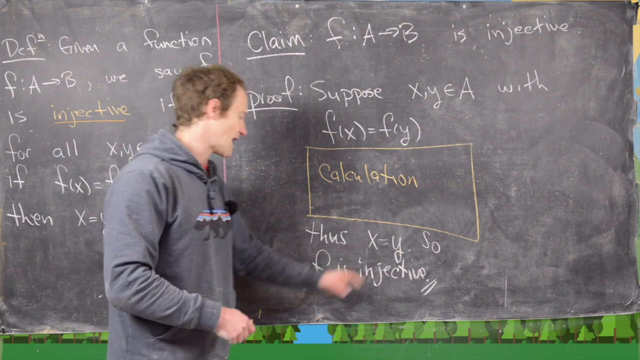 a with f of x equals f of y, and then you'll take this equation f of x equals f of y and you'll do some calculations on this equation until you get down here to this point that x equals y, and then that tells you that f is. 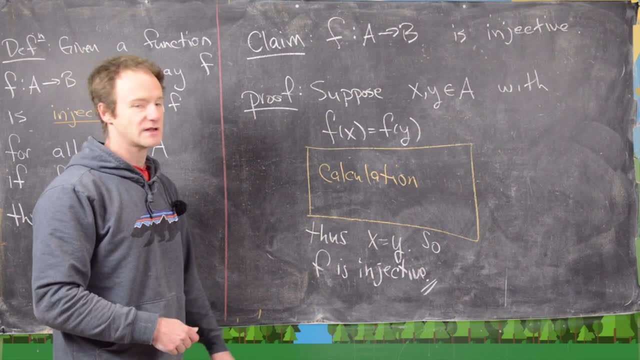 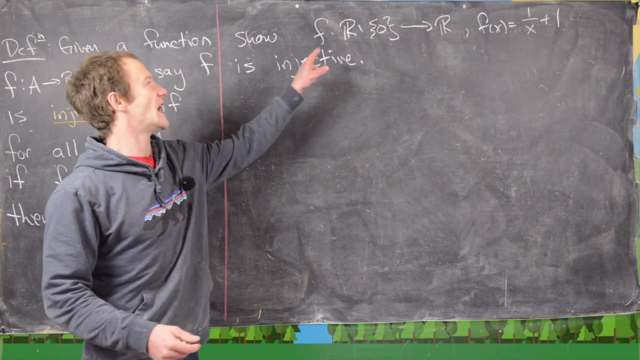 injective and that's all there is to it. Okay, I'll clean up the board and we'll look at some examples. Okay, so we want to show the following: function is injective, So let's define it with the domain of r minus the number zero and then the. 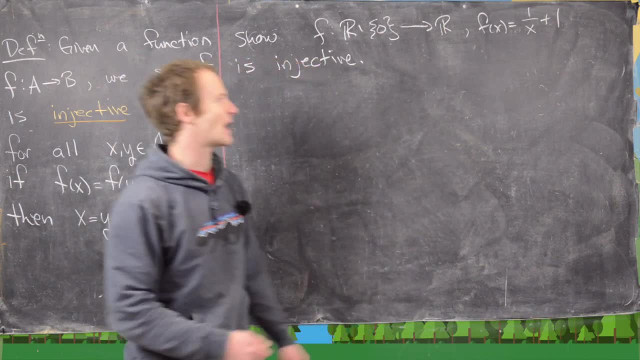 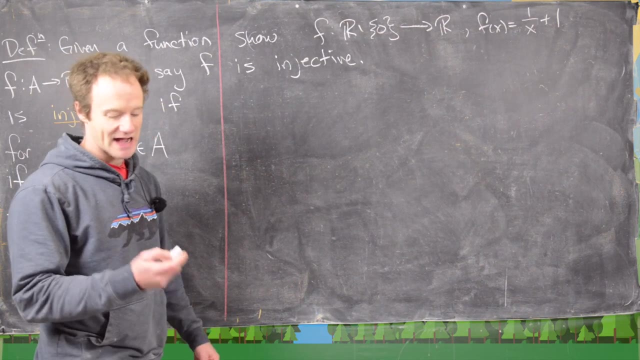 range of the number zero, and then the range of the number zero and then the is just all real numbers. And so f of x is defined by 1 over x plus 1.. So that makes it clear why we had to exclude 0 from the domain. We want to show that guy's injective. Okay, so we're going to. 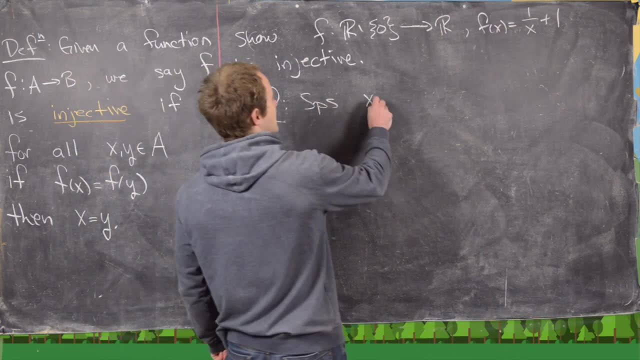 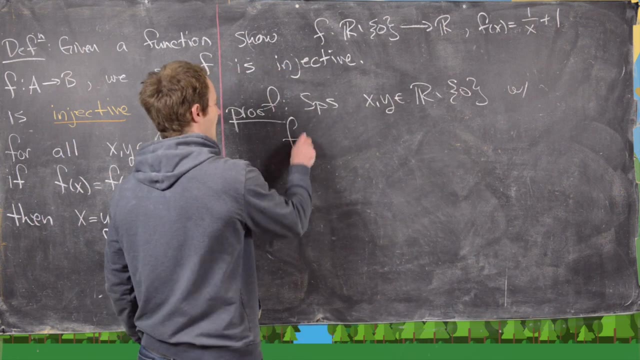 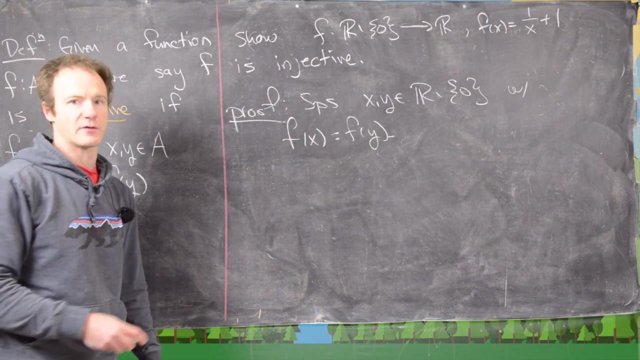 follow our proof outline. So let's suppose that x and y are in the domain. So that's r minus 0, with f of x equals f of y. Great, But then we can apply our formula that we know for f of x minus f of y. 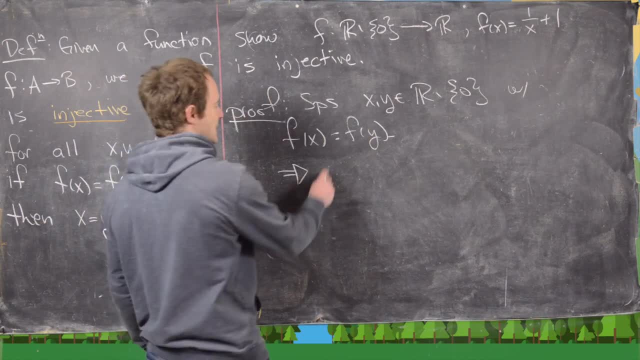 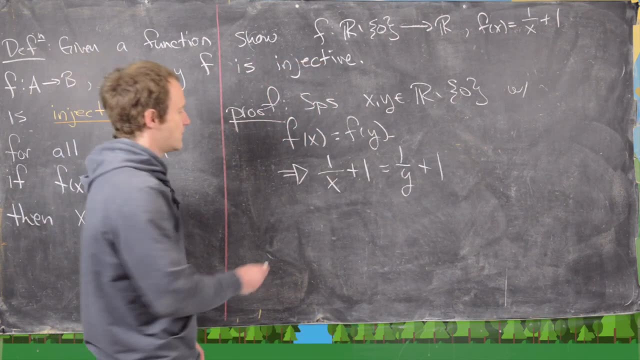 So what that tells us? sorry, f of x equals f of y. that tells us that 1 over x plus 1 equals 1 over y plus 1.. Great, But then that immediately follows that 1 over x equals 1 over y. But then, 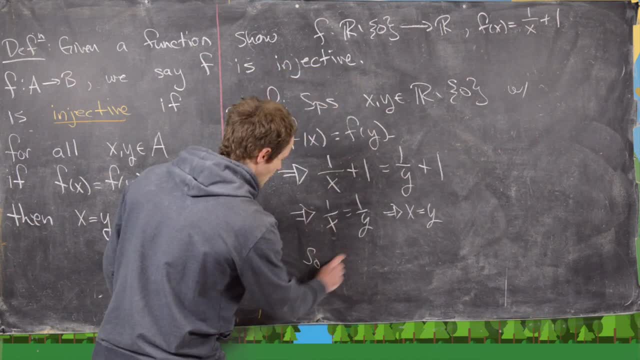 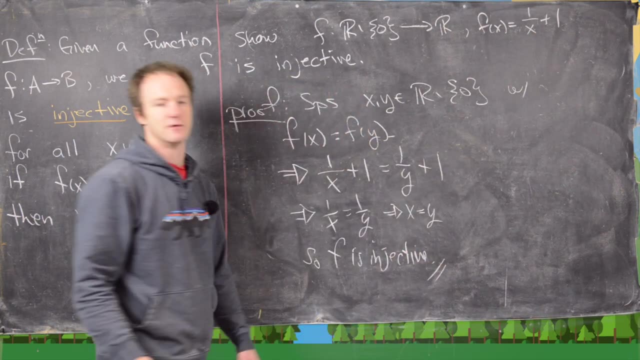 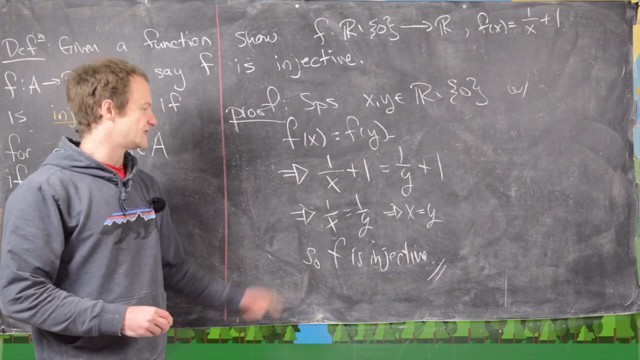 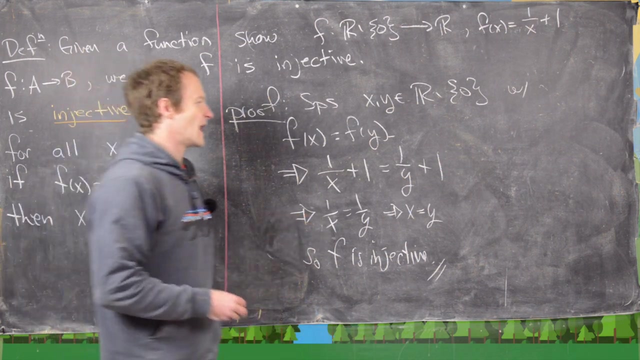 also, that follows that x equals y, So f is injective. And that finishes our proof. And before we move on to the next example, I want to make an important point about presenting proofs on a chalkboard and talking them out verbally versus writing them down like for a homework exercise. And if you were to do 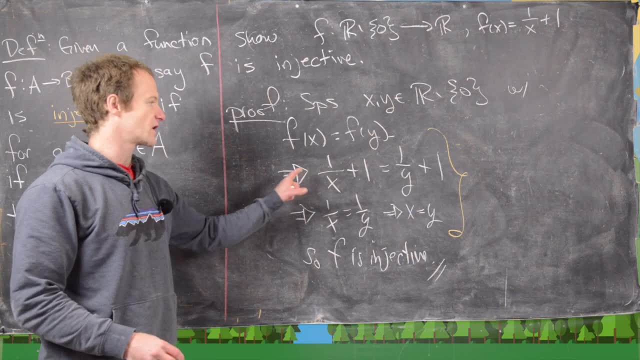 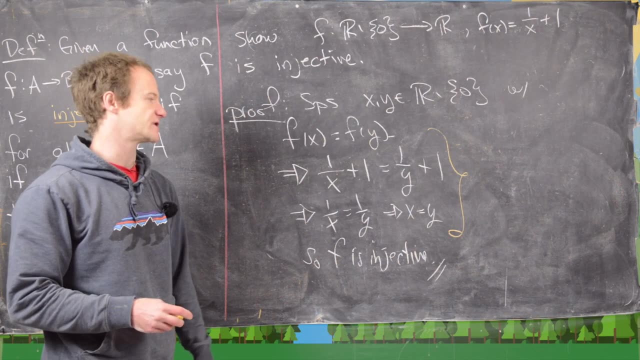 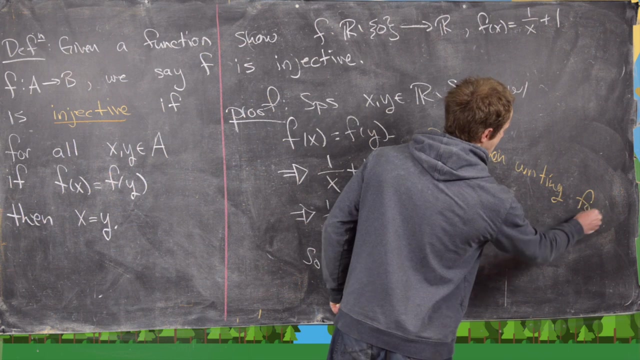 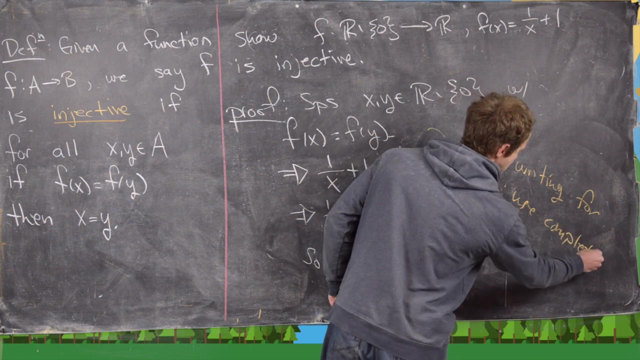 such an exercise in homework, you would replace this shorthand that's very common for use on the chalkboard and very appropriate for use on the chalkboard with words. So in other words, when writing for homework here, you would use complete sentences And not this kind of. 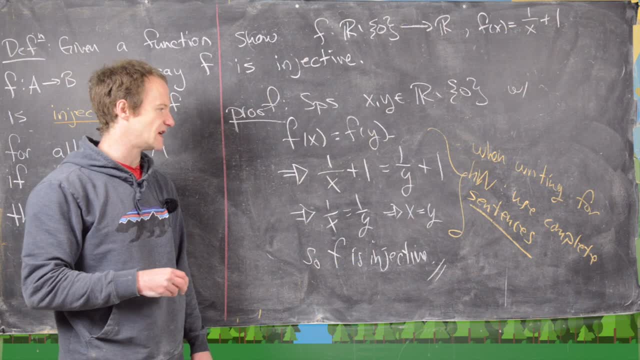 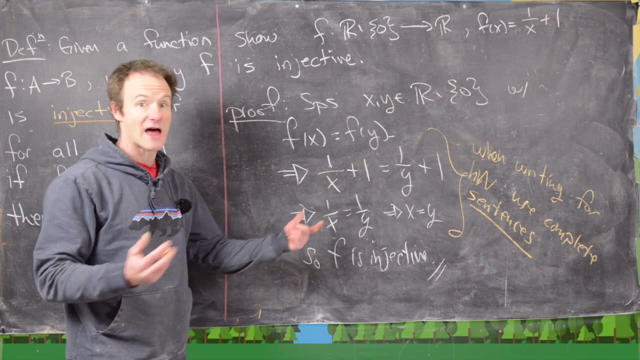 shorthand, And so this is something that's really important to keep in mind: that presentation of a proof on a chalkboard and writing it on a chalkboard is very appropriate for using complete sentences. So if you're writing it down for homework or for a math paper that you're writing, or 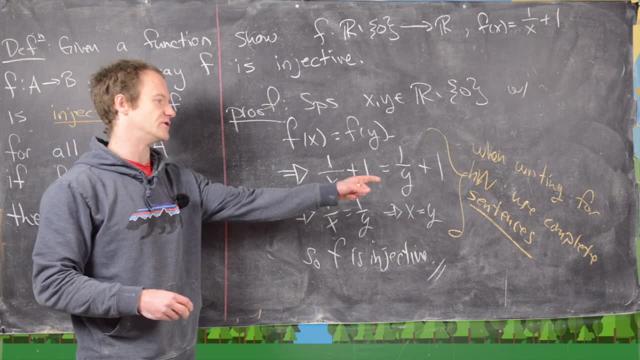 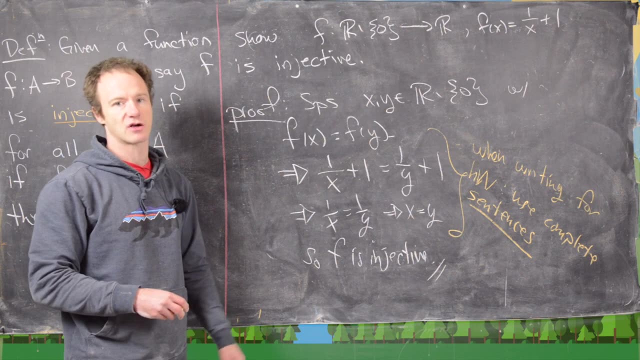 anything like that is a different beast altogether. And you want to use complete sentences over there, whereas you can say the complete sentences to your audience when you're writing it on a chalkboard. Okay, I'm going to clean up the board and then we'll do another example. 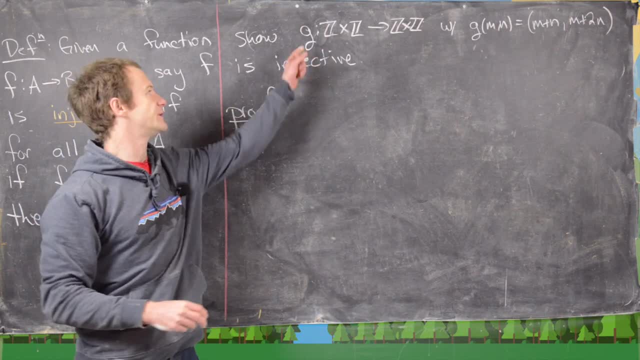 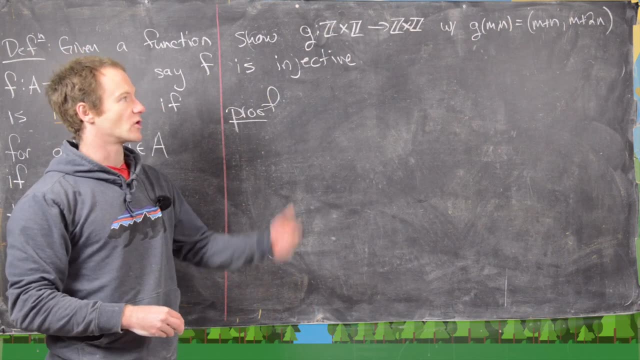 Okay. So for our next example, we'll look at the following function. So we've got this function: g from z cross z to z cross z. It's given by g of mn equals 1 over x plus 1.. And it's given by the ordered pair m plus n, m plus 2n. So we're going to follow the same outline that we 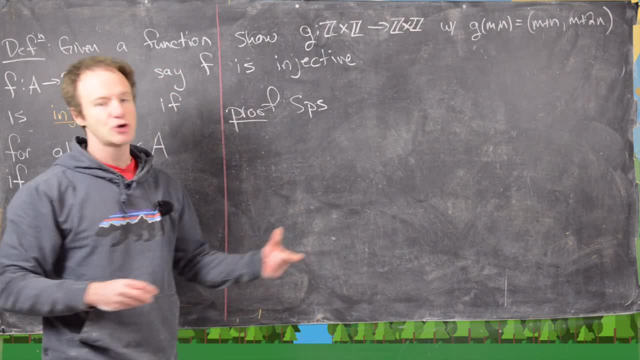 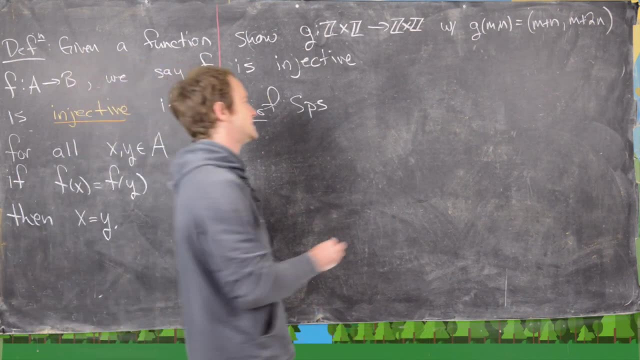 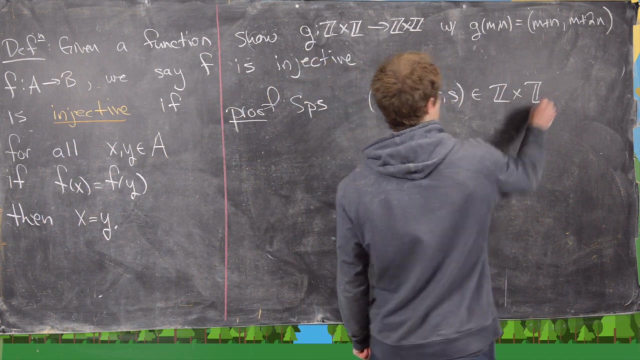 did before. So let's suppose that we have two elements of the domain. So last time we wrote them as x and y, but maybe we want to choose something different because our domain is z cross z. So let's choose m comma n and maybe r comma s. Those are both elements of our domain. 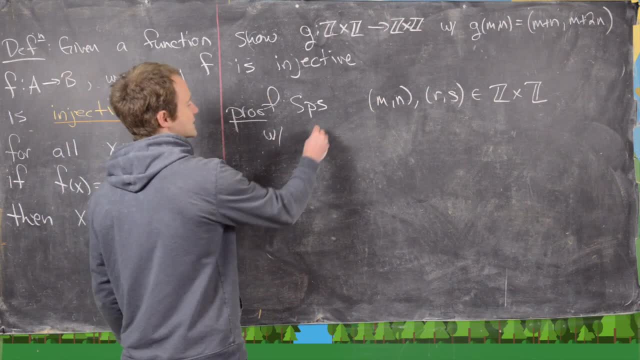 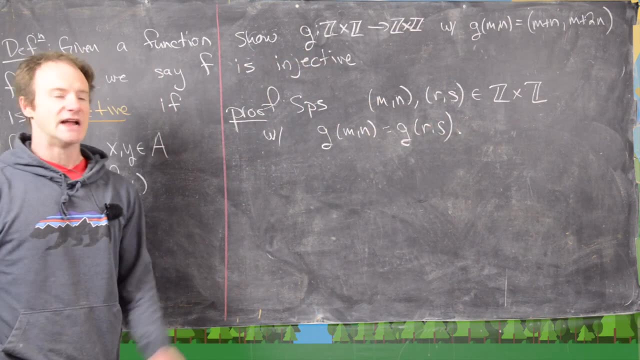 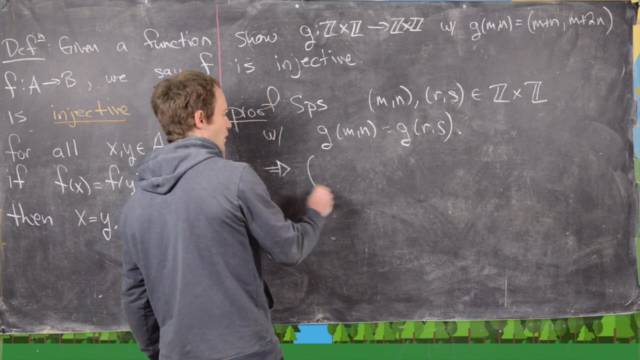 z cross z, And they satisfy this rule that g of mn equals g of mn. So we're going to follow the formula g of rs. Great, And so from there we can apply the formula that defines g And that tells us that we have the ordered pair m plus n, and then m plus 2n equals the ordered. 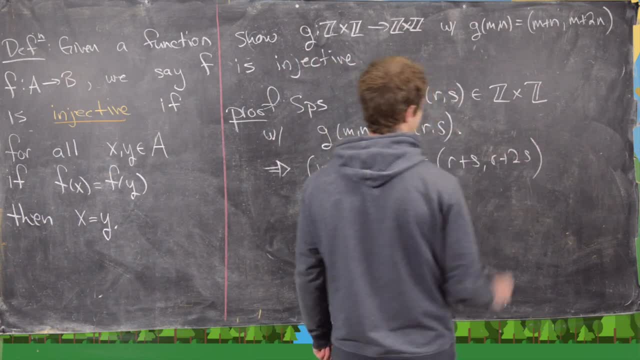 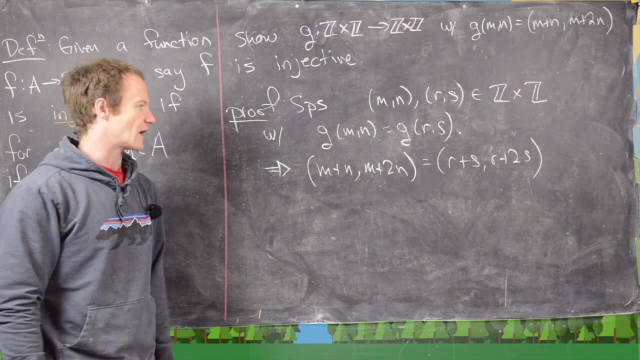 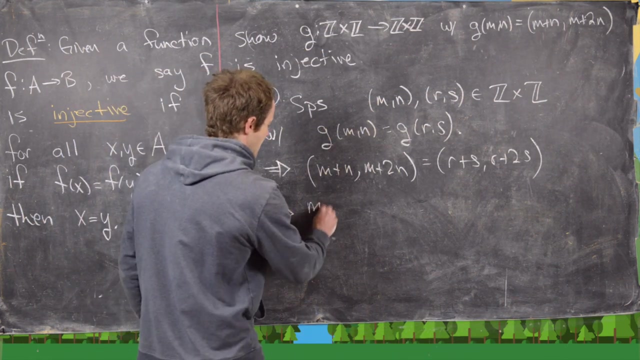 pair r plus s, r plus 2s, And that's just given by this left-hand side and this right-hand side. But then let's recall that ordered pairs are equal if, and only if, r plus 2s equals, their entries are equal. So that gives us two equations: m plus n equals r plus s and m plus